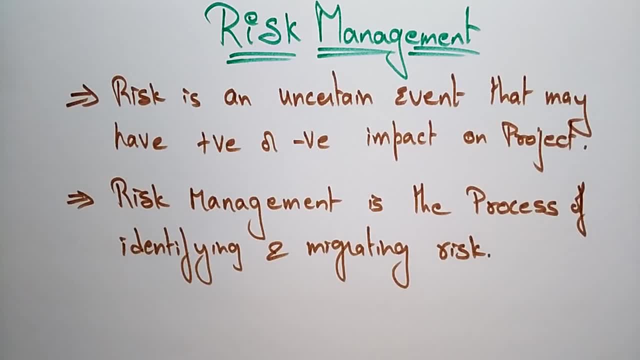 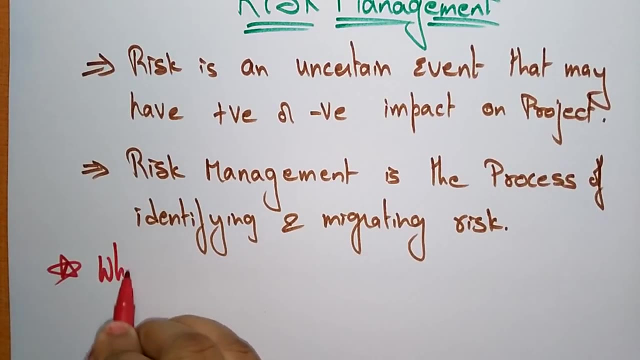 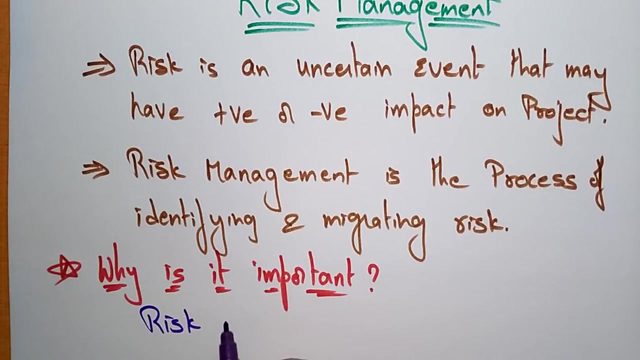 techniques to solve the risk, to identify the risk and to solve the risk so that you call it as risk management. so why is it important? why this risk management is important? let me write that. why is it important? is it necessary to know about the risk in the project? yes, it is necessary- the risk effects it affects. 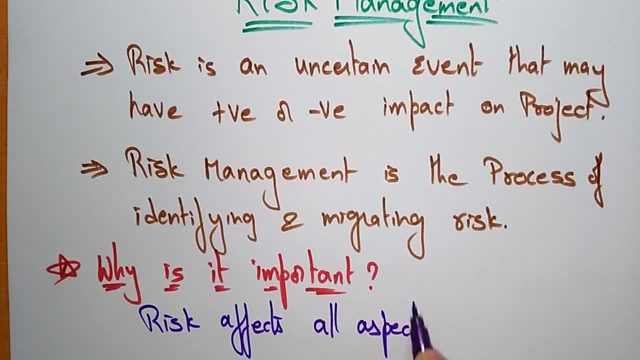 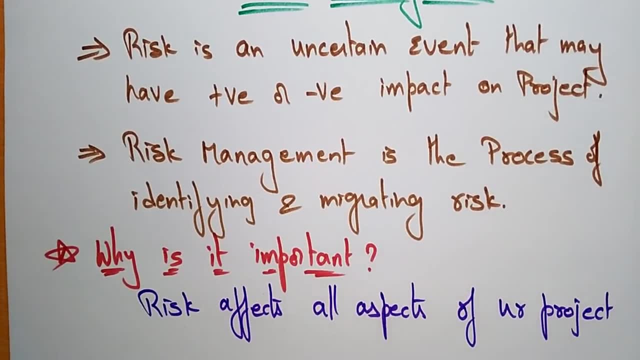 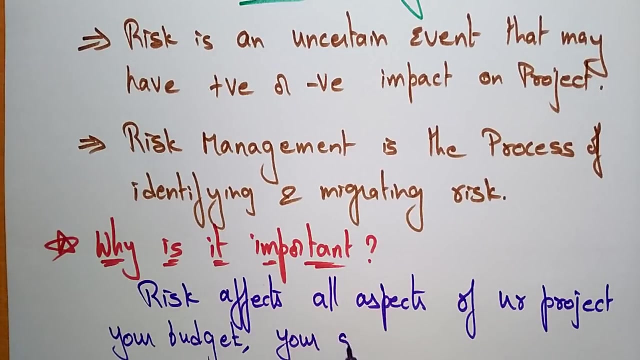 all aspects, all aspects of your project. so it affects all aspects, all the fields, all the modules of your project. that is your budget, your budget. it is going to be affect your budget. it is going to be affect your schedule. sometimes it may. with the hell with this risk management. 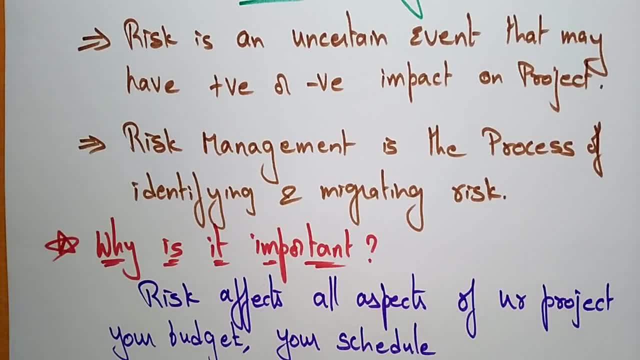 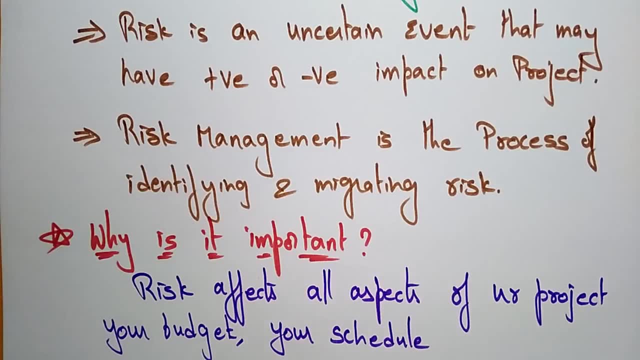 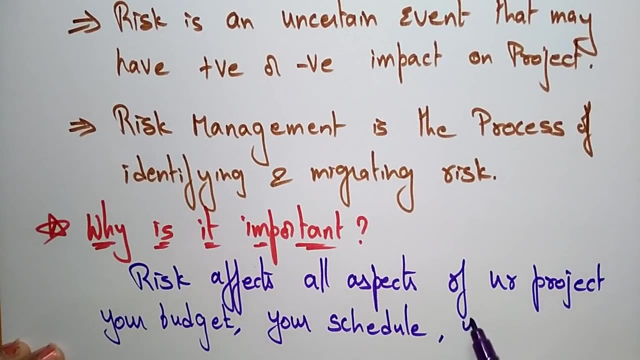 the projector has to be extended, the schedule will be changed. okay, in your budget it may. sometimes it may leads to high rather than your expectations. from your expectations it leads to high. your budget, your schedule, your scope, everything will be affected. so that's why you have to be managed at risk. 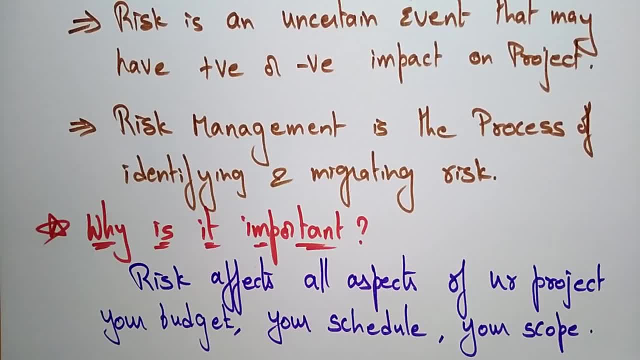 carefully. the risk management is a process of identifying and migrating the risk. so we, if you want to develop any project, you have to know about the risk management. also. is it if you say, is it important? yes, it is important because it affects all your aspects of your project, like your budget, your schedule and your scope. 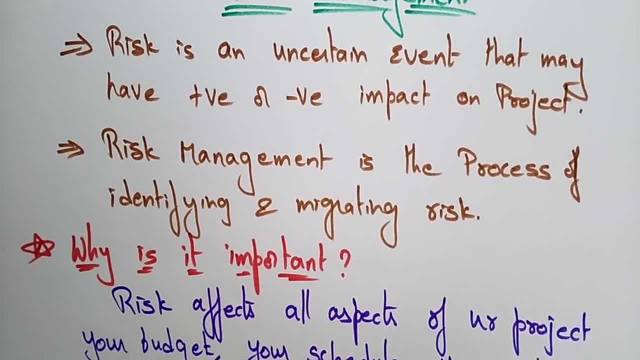 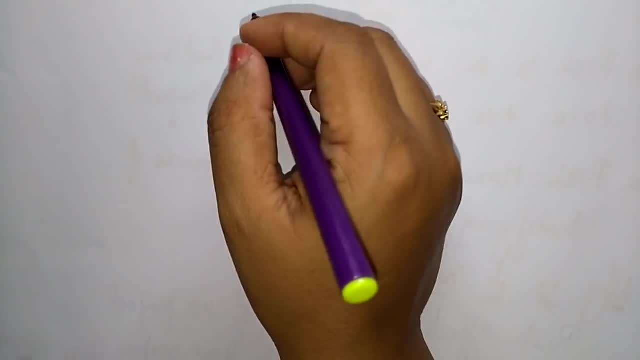 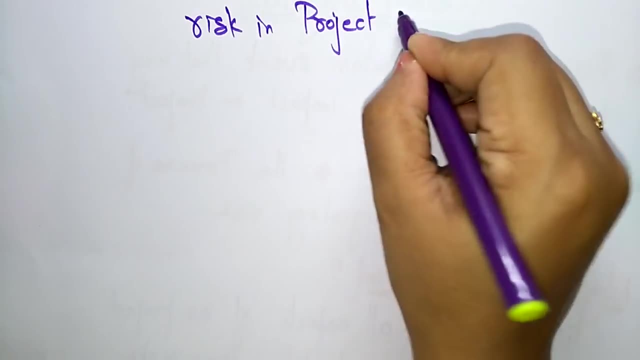 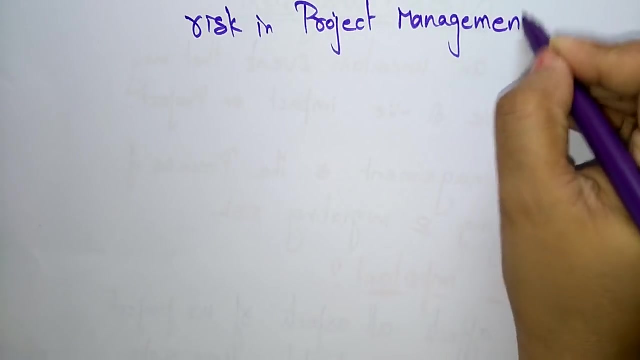 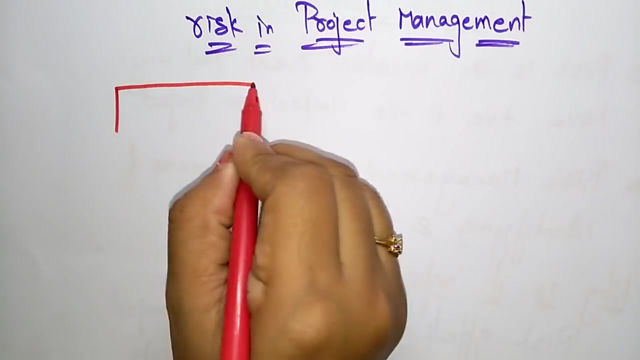 so increasing the probability of positive event. it reduces the occurrence of negative event also. so what does it include? what risk management will be included? now let us see risk in project management. so what are the risks that are involved in the project management? project risk in project management? so there are.